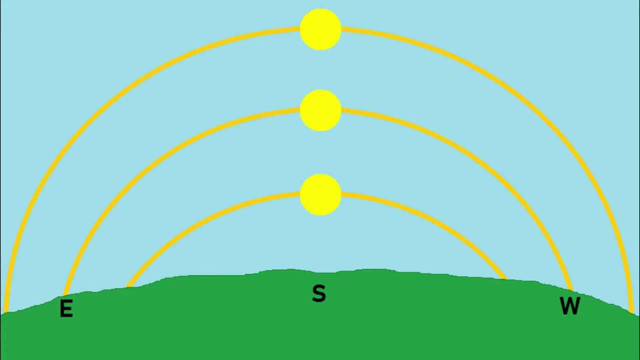 The sun would also follow a corresponding path in the sky further to the north or south, and setting further to the north or south of west, The daily change in position seems to happen faster towards the midpoint and appears to slow down at either end of the cycle. 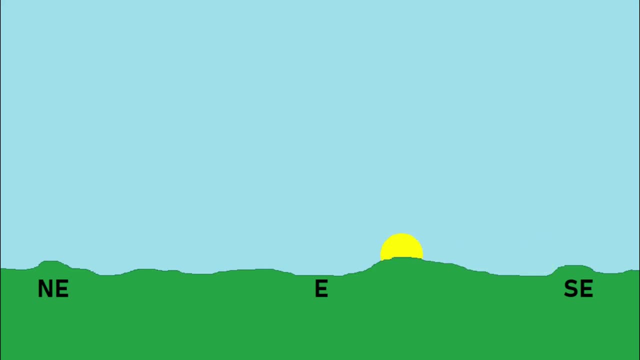 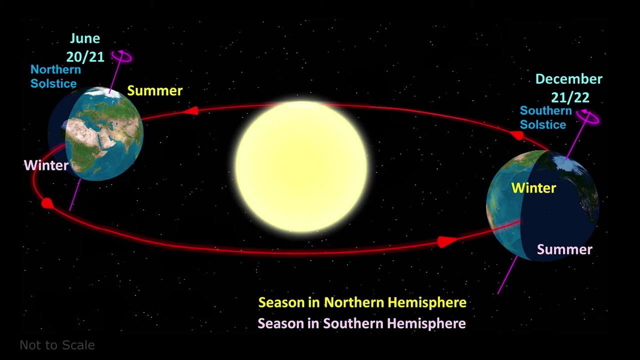 The two maximum positions are called solstices, from the Latin for sun and stand still, and they can be distinguished as the northern solstice and the southern solstice. In the northern hemisphere, the northern solstice is more commonly referred to as the summer solstice. 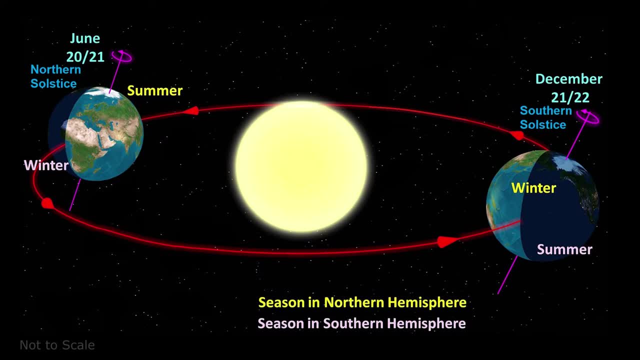 and the southern solstice is called the winter solstice, But in the southern hemisphere it is the southern solstice that occurs in summer and the northern solstice that occurs in winter. The northern solstice occurs around June 21st and the southern solstice around December 21st. 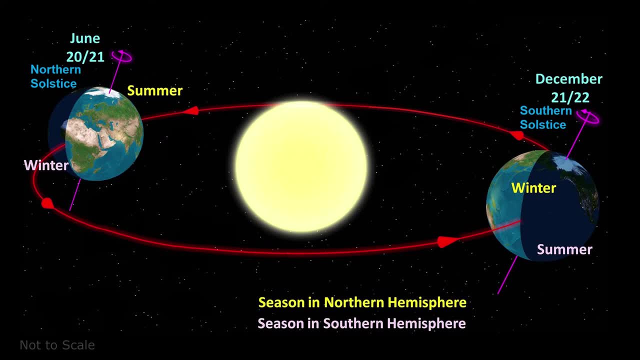 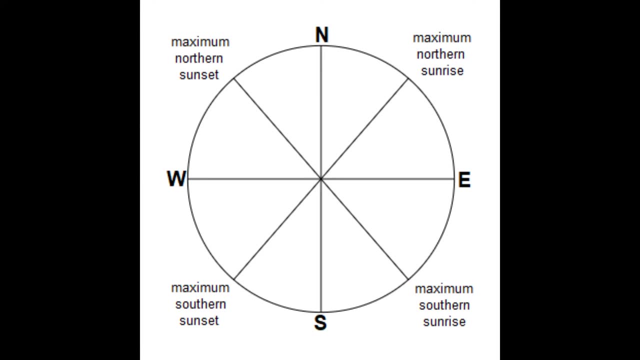 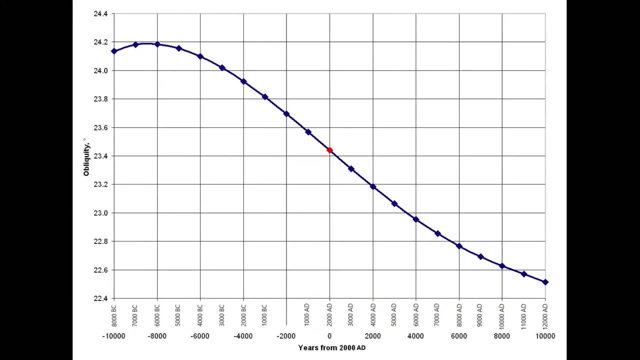 although the exact date changes because of fractional calendar adjustments, Determining the maximum position of the sun on the horizon is not the same as determining the exact date of a solstice, because there is so little observable change as the exact time nears. The tilt of the earth has been decreasing over the last few thousand years. 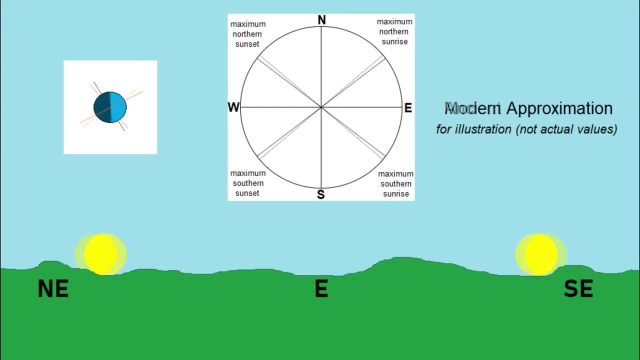 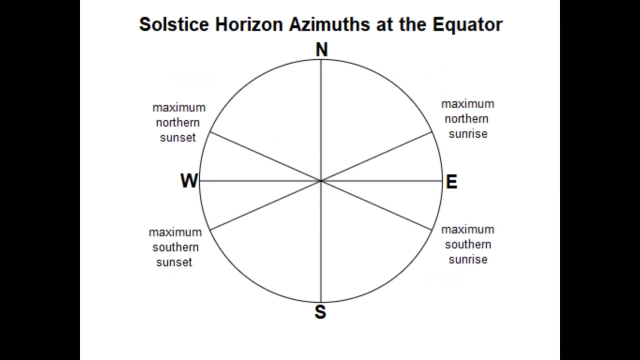 so that today the maximum positions are slightly less extreme than in the past. Towards the equator, the sun rises at an angle that is more perpendicular to the horizon, and the angle between where it rises at each solstice is not very wide. Near the equator, the sun also passes directly overhead twice each year. 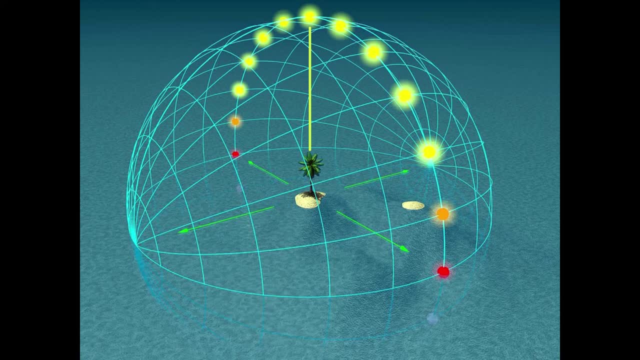 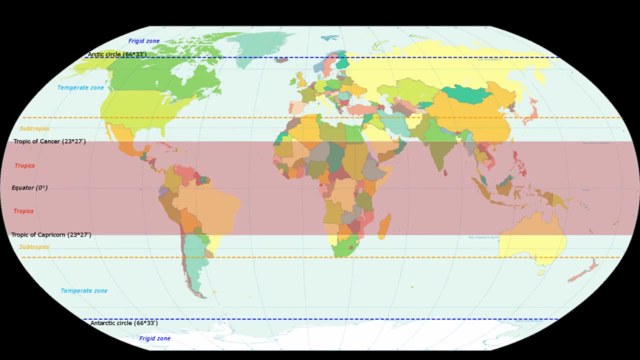 as it goes between the northern and southern maximums. When this happens, it is known as a zenith passage. The imaginary lines that define the tropics are the last positions to the north or south of the equator that the sun can pass directly overhead, and at those latitudes, 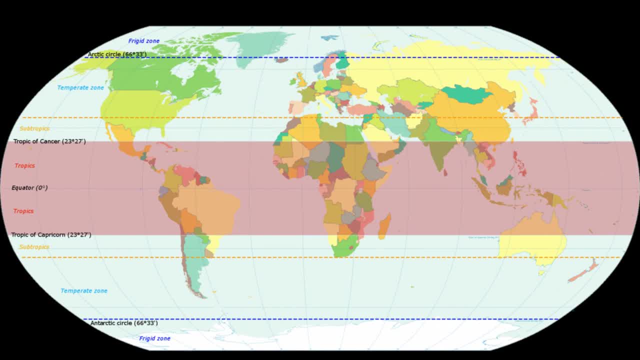 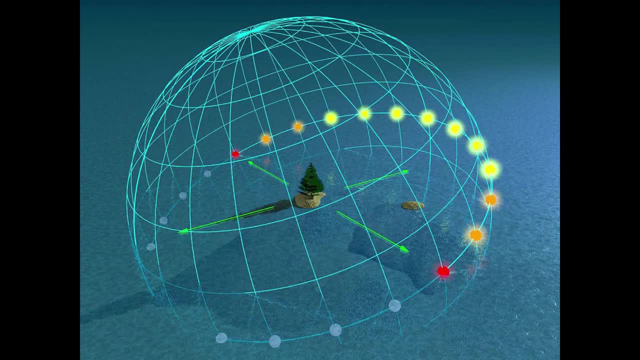 the zenith passage occurs just once a year. at the solstices, The sun rises at an angle that is more perpendicular to the horizon than at the equator. The sun rises at sharper angles relative to the horizon the further north or south a location is positioned on the earth. 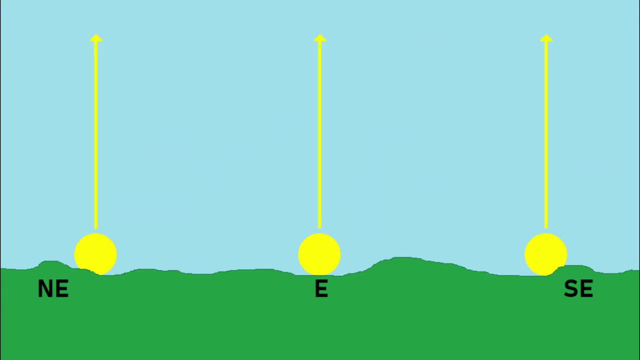 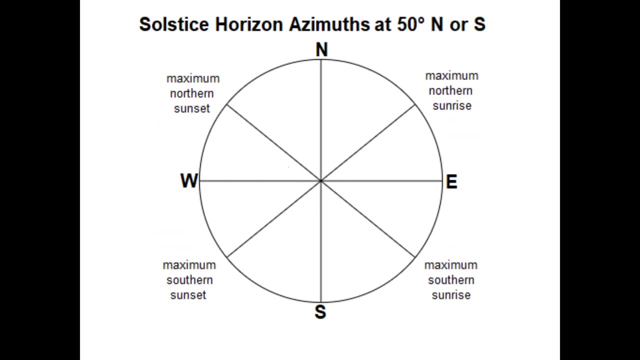 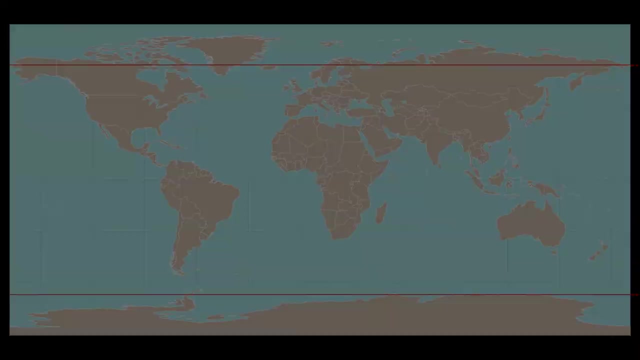 In the northern hemisphere the sun angles to the south, and in the southern hemisphere it angles to the north. The change in sunrise and sunset positions on the horizon become much more extreme Beyond the latitudes of the arctic and antarctic circles. 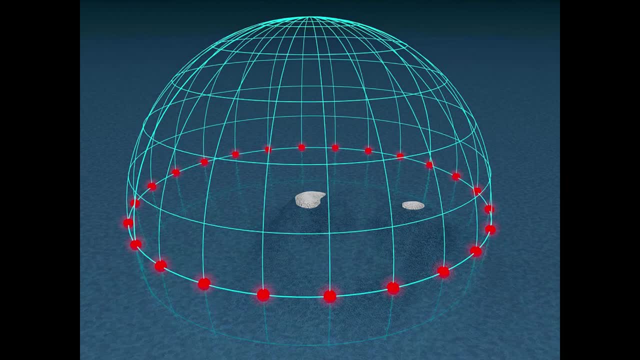 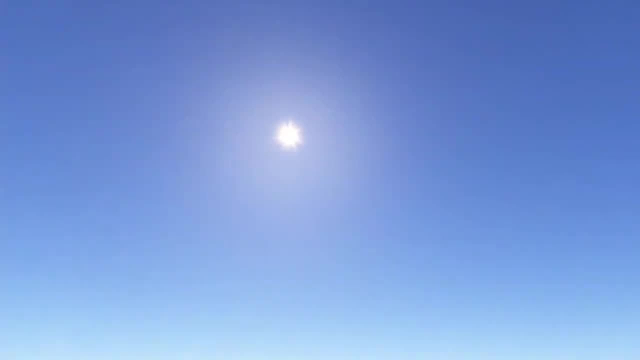 the extremes reach a point where, at one maximum, the sun never comes over the horizon at all and at the other, it never sets, instead tracing a great circle around the sky, closer to the horizon at midnight and a bit higher at midday, but always visible. 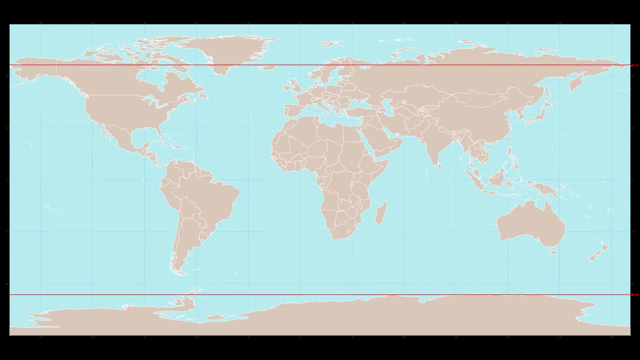 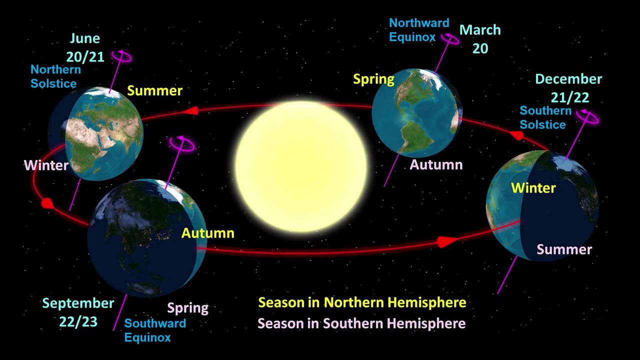 The number of days this occurs increases towards the poles. In modern times, we have labeled the midpoints between solstices as the equinoxes. when the earth reaches the two points in its orbit where it is oriented exactly sideways to the sun. 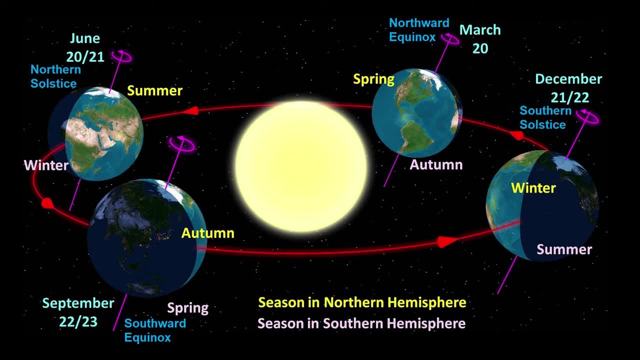 The vernal equinox occurs around March 21st and the autumnal equinox around September 21st. They are often referred to as the spring and fall or autumn equinoxes, but since the seasons are opposite in the northern and southern hemispheres, 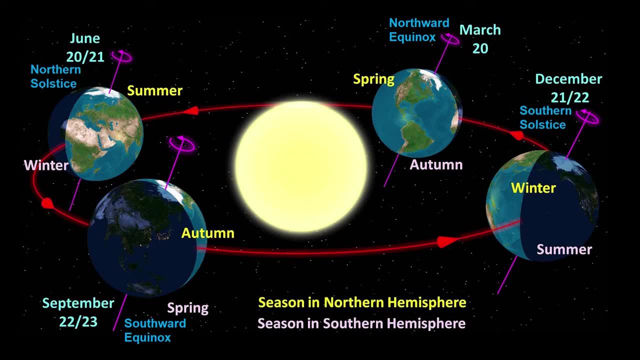 they can also be distinguished universally as the northward equinox and the southward equinox, as the apparent position of the sun is moving in one direction or the other, as it passes due east and west, and the amount of daylight becomes more or less equal. briefly, 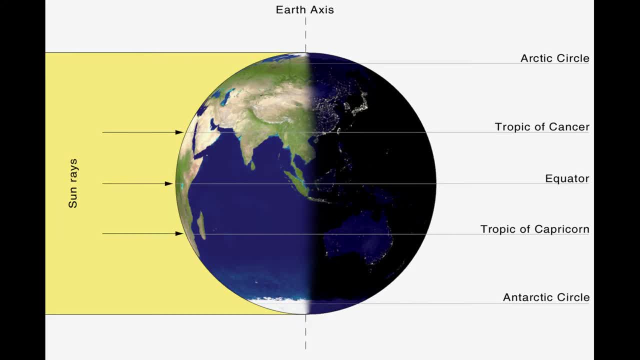 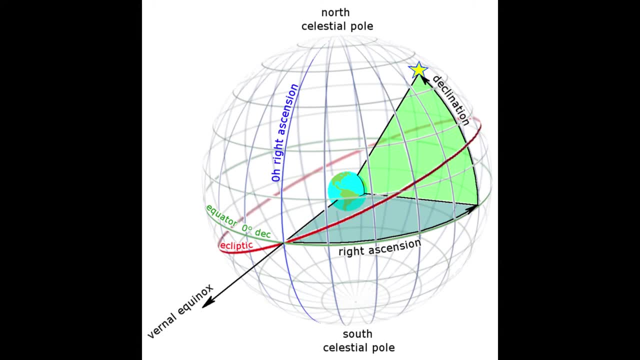 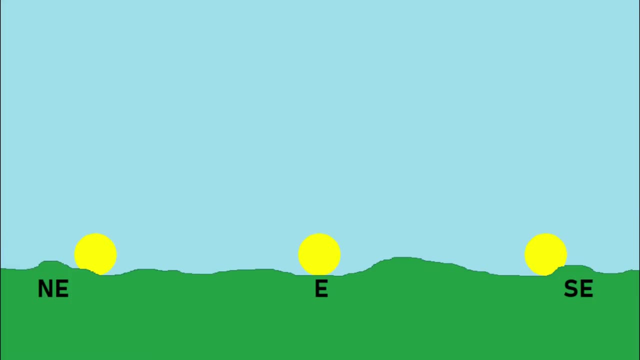 before beginning to increase or decrease again. Our modern concept of equinox is based on measurements of declination against coordinates. In the past it is possible that there was some interest in a similar concept of estimating a midpoint in time between solstices or estimating a rough middle position along an uneven horizon. 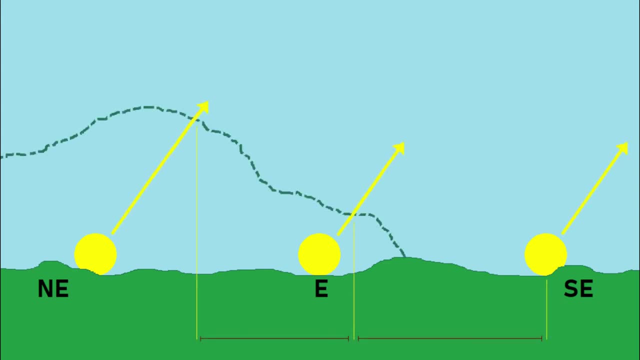 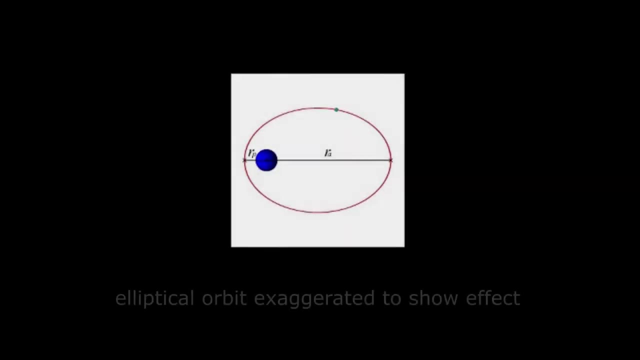 but this is not as straightforward as it might seem. The equinoxes occur roughly halfway between the solstices in time, but not exactly, because the Earth moves slightly faster and slower at different points along an orbit that is not quite a perfect circle. 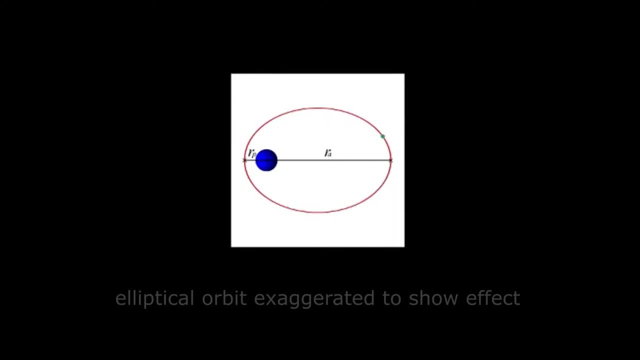 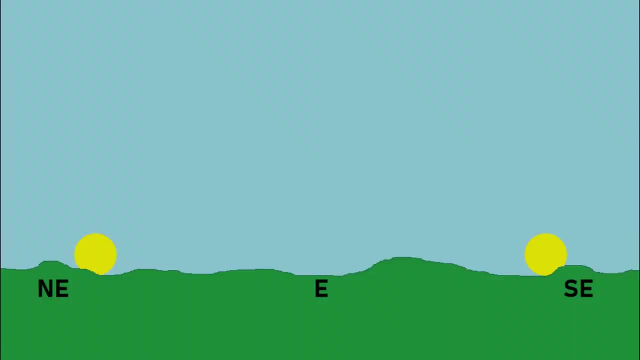 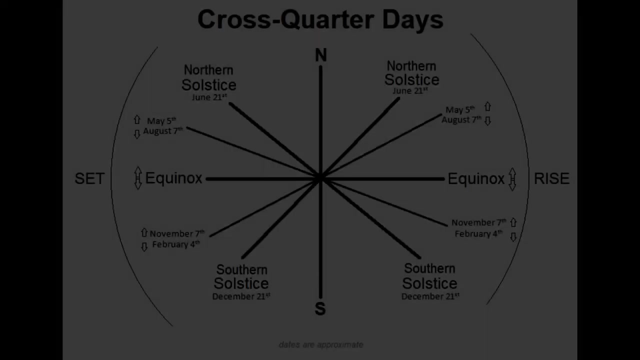 Even counting the days between solstices to find an approximate midpoint has problems, as determining the exact day of a solstice is difficult because the position of the sun seems to change very little for several days at each maximum. Other methods for dividing the year further by time intervals: